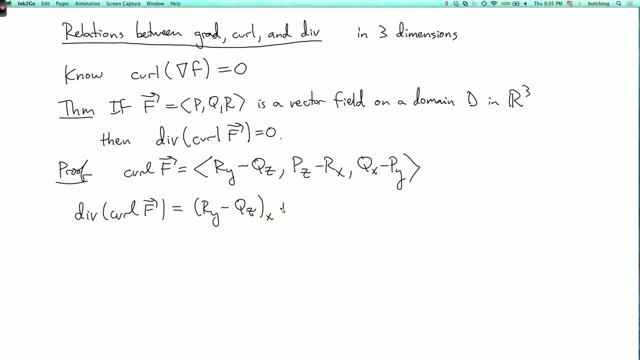 she's V a into the second term, which is a y and differentiated with respect to x. Then I add the second term differentiated with respect to y and then the third term differentiated with respect to z. So this is Ryx minus Qzyx plus Pzy minus Rxy. 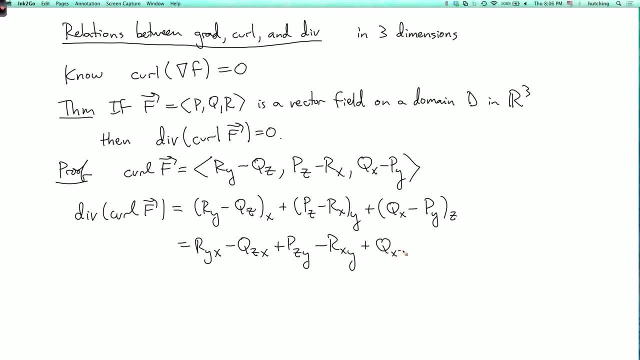 plus Qxz minus рыxy, plus Qzyx plus Ryx minus PYZ. And now I see if I can cancel stuff. So here I have an RYX and there I have a minus RXY. So by Clairaut's theorem I can cancel those. 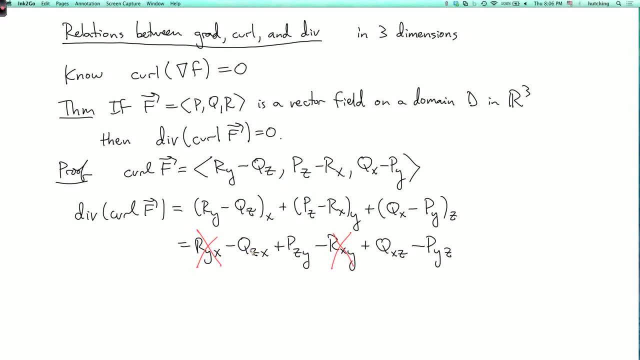 And here I have a minus QZX and here I have a plus QXZ. so by Clairaut's theorem I can cancel those. And here I have a plus PZY and a minus PYZ. so by Clairaut's theorem I can cancel those two, And now there's nothing left. 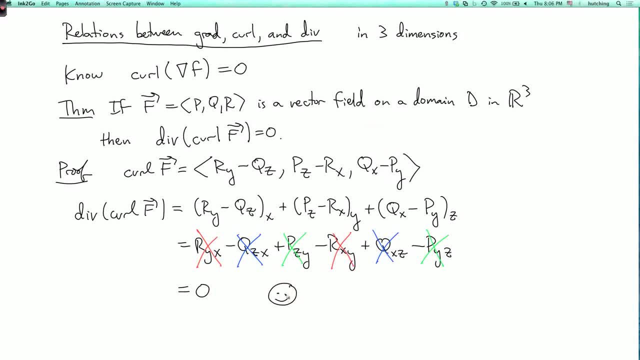 so I have zero and we're done. So it's not totally obvious, but a straightforward calculation. And then it's a fact that you can sort of go the other way. So this says that if a vector field is the curl of something, then its divergence is zero. 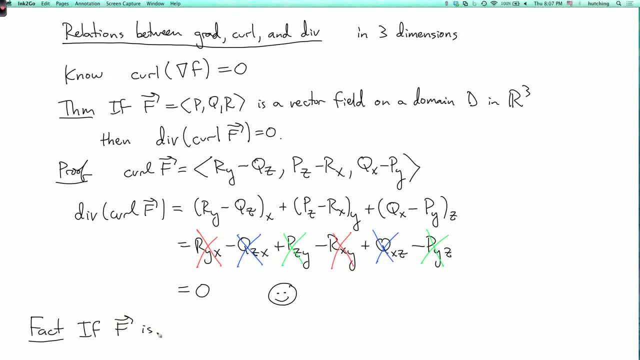 So if F is a vector field on all of R3, if there are certain kinds of holes, this won't work. But if it's a vector field on all of R3 and the divergence of F equals zero everywhere, then F is the curl. 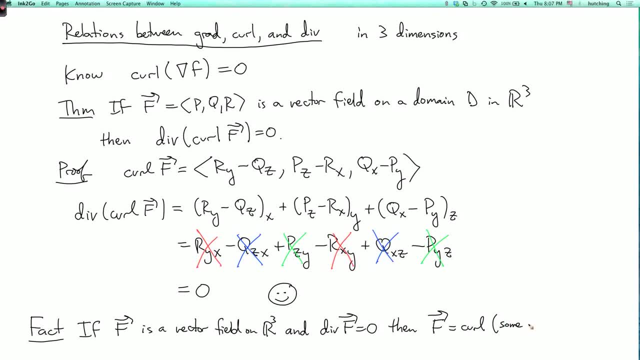 of some other vector field. This is really beyond the scope of this course. I'm just mentioning it for amusement. So it's sort of analogous to the curl of the gradient of F business. So we know that if on all of R3, if the curl of a vector field is zero, then it's the. 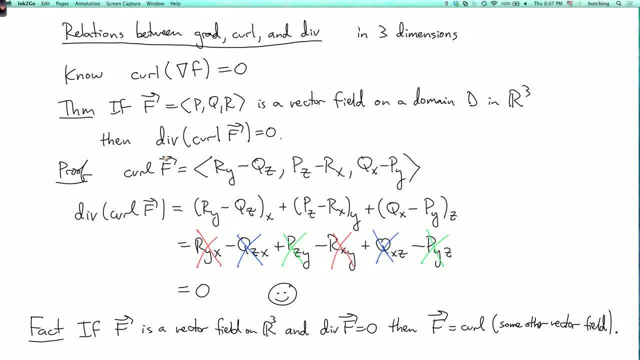 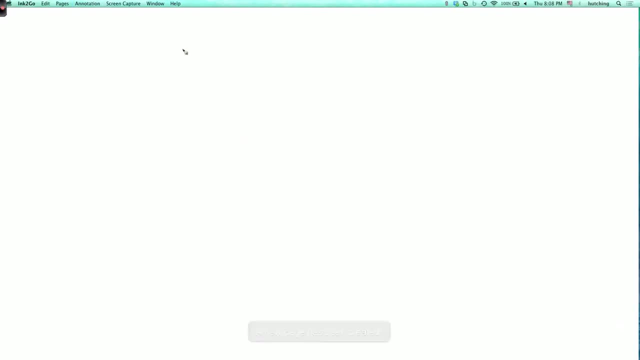 gradient of something. And we also know- at least this fact says- that if you have a vector field and its divergence is zero, then it's the curl of something. Okay, so let's sum this up in a chart. So, if you have a function, 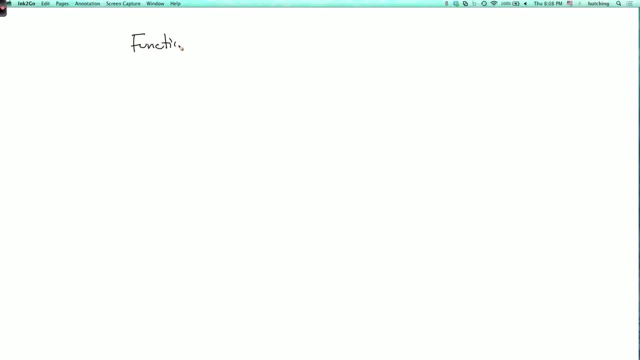 you can take its gradient to get a vector field. Now, if you have any vector field, you can take its curl to get another vector field. And also, if you have any vector field, you can take its divergence to get a function again. Now, if you do two of these operations in succession, you get zero. 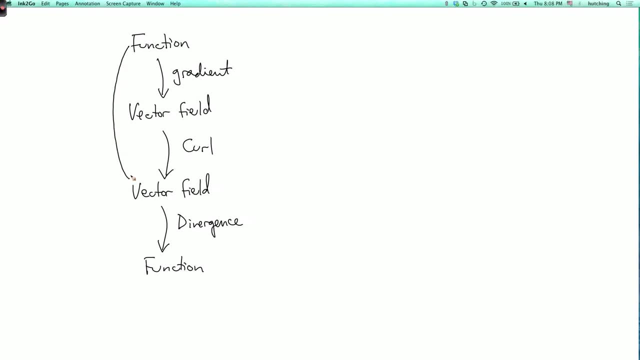 So if you take the gradient of something and then take the curl of it, you get zero. So this is a restatement of the fact that the curl of a conservative vector field is zero. And we just saw on the previous page that if you take a vector field and take its curl and then take the divergence of that, then that's also 0.. 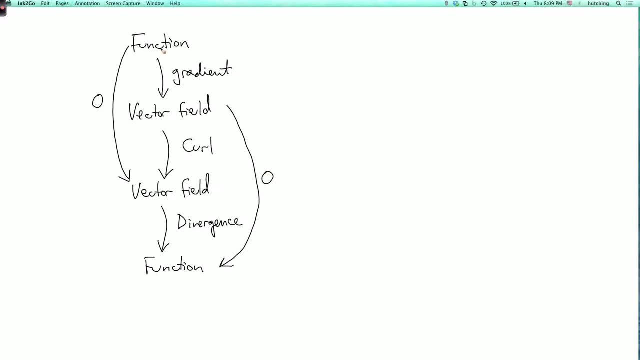 There's one last thing we might try to do, which is take a function, take its gradient and then skip the curl part and take its divergence, And this is not 0. So if f is a function on R3, what I'm about to say actually makes sense in any number of dimensions. 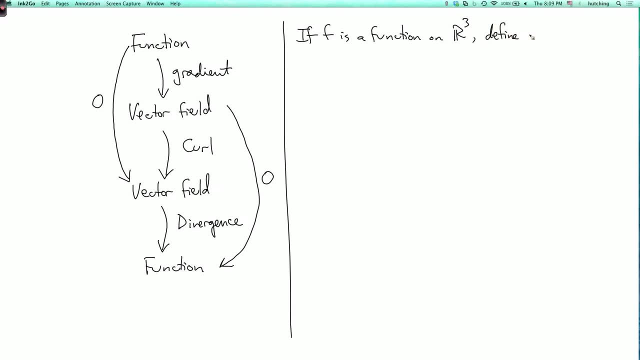 One defines the Laplacian. So this is sometimes denoted by a right-side-up triangle, but sometimes denoted by del squared f. So the del squared f is the divergence of the gradient of f. We could also write this as del dot del f. 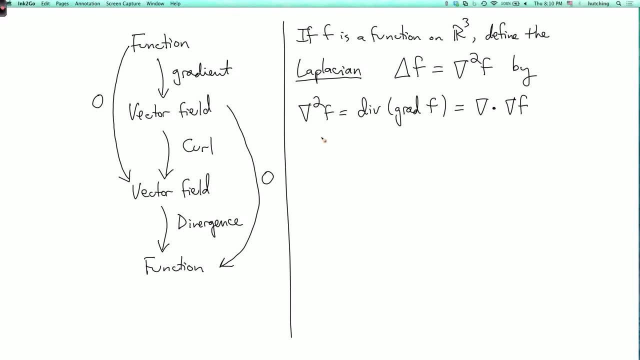 And if you write that out in components and work out what it is, well remember, the gradient of f is the vector field, fx, fy, fc, And so the divergence of this is when you take the derivative of the first component with respect to x, so we get fxx. 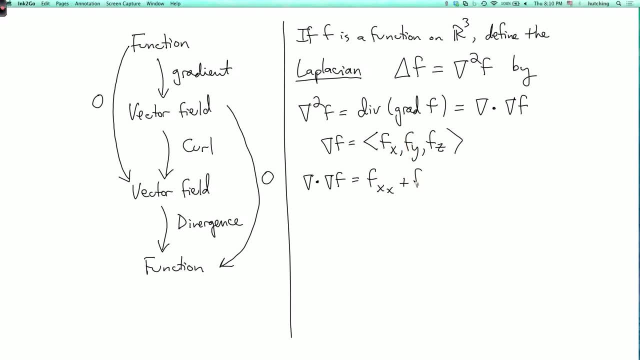 And then you add the derivative of the second component with respect to y, so it's fy y. And then, finally, you add the derivative of the third component with respect to z, so it's fzz. So this is the Laplacian.